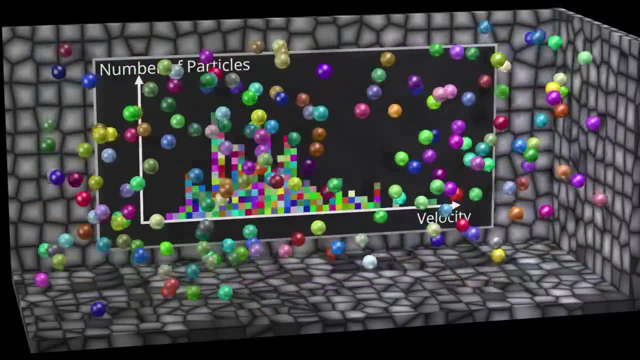 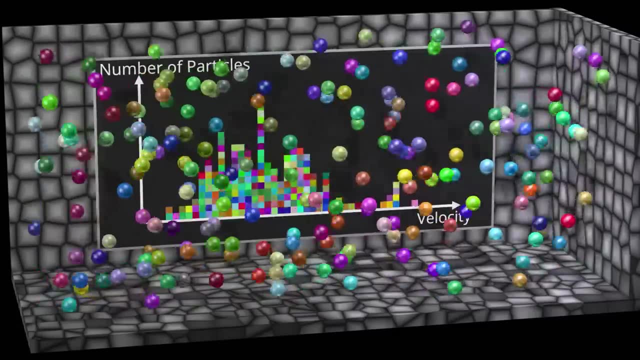 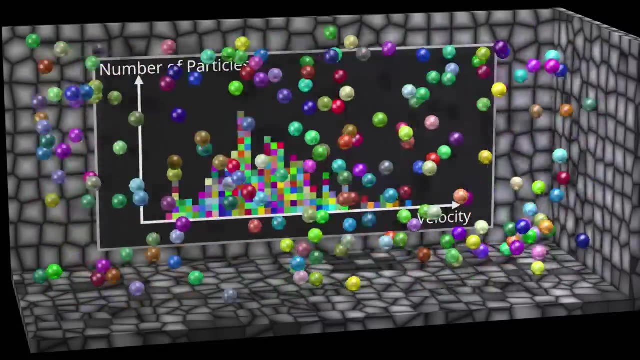 In the graph, the velocity of each particle is rounded to the appropriate number of digits so that all the squares neatly fit into columns. This system quickly reaches what we call thermodynamic equilibrium, And the graph for the velocity distribution ends up looking as shown: 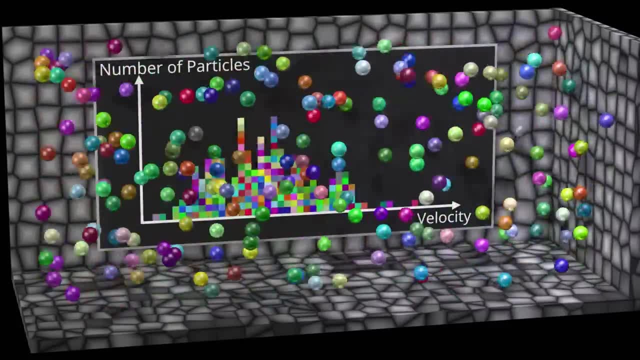 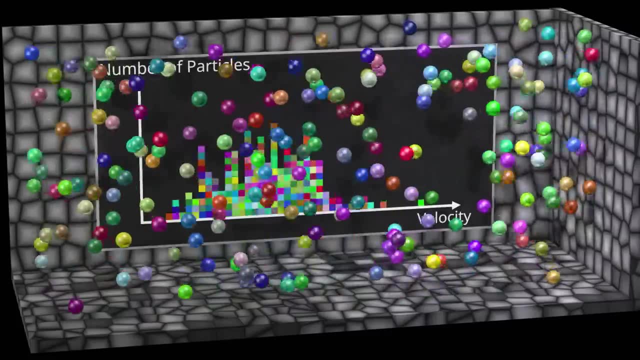 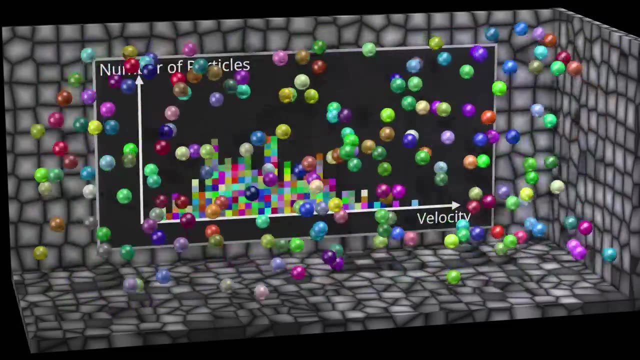 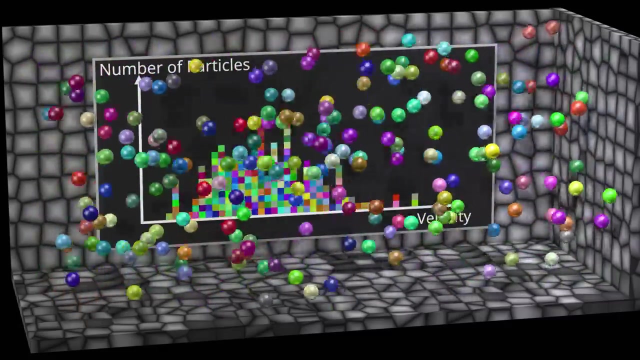 A system is in thermodynamic equilibrium when the entropy of the system has reached its maximum possible value. given the constraints of the system, Entropy is a measure of how many different ways something can occur. There are only a small number of ways in which all the energy can be given to only a few particles, and hence the situation at the beginning had a smaller entropy. 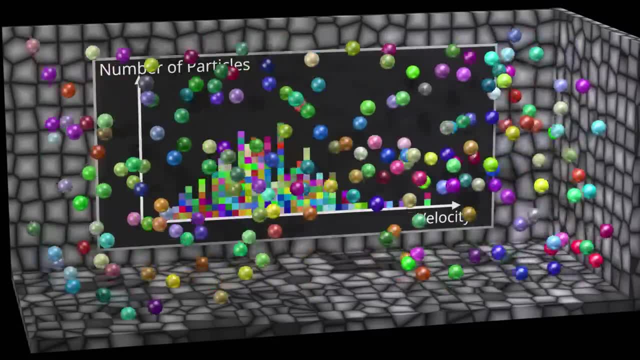 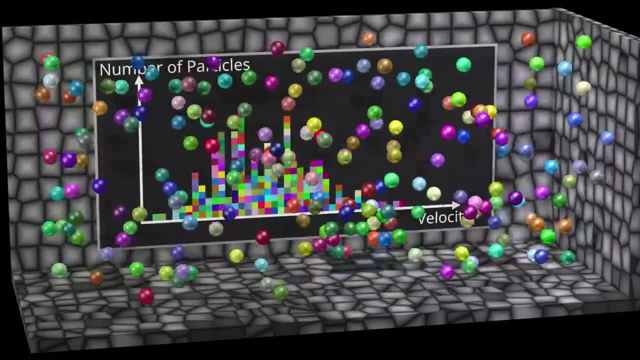 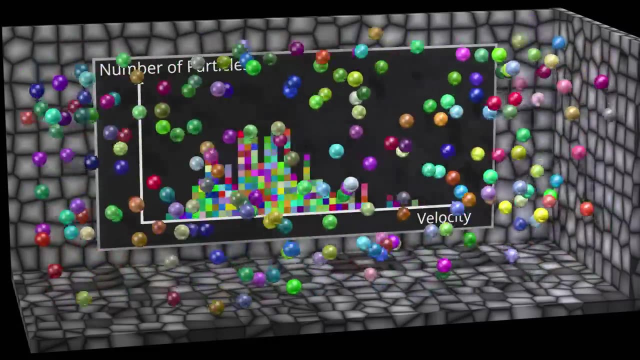 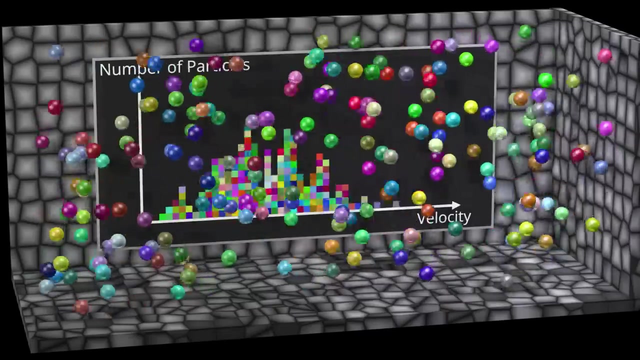 There is a much larger number of ways in which the energy can be dispersed as shown, and hence this situation has a higher entropy. If all the particles hypothetically had the exact same energy, then this would have a lower entropy because there is a smaller number of different ways in which all the particles can have the exact same velocity magnitude. 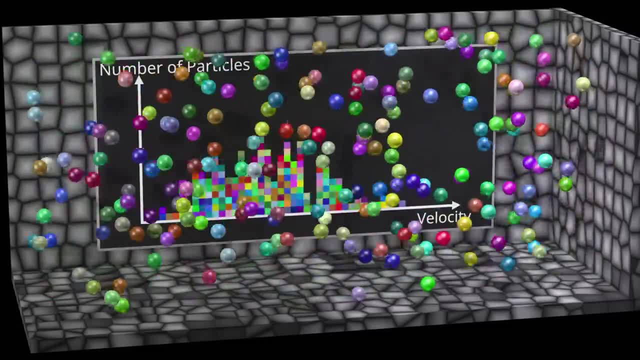 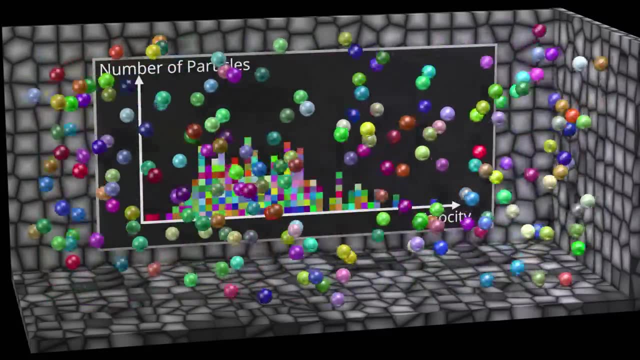 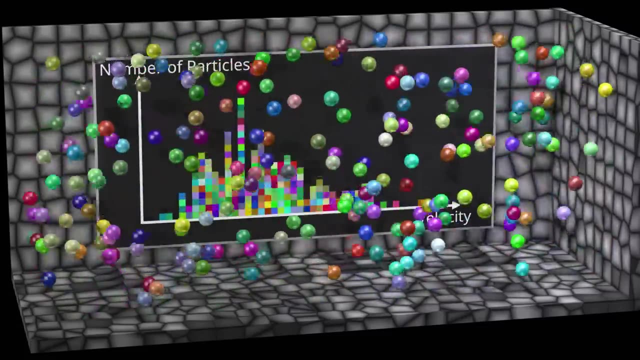 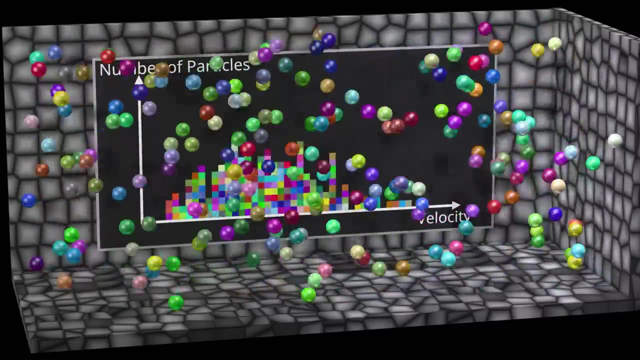 There is a much larger number of ways in which the velocity magnitudes can be dispersed on the graph, as shown, and this velocity distribution is what we get when the entropy is at its maximum for this given temperature. In this simulation, all the particles are represented as spheres interacting through perfectly elastic collisions. 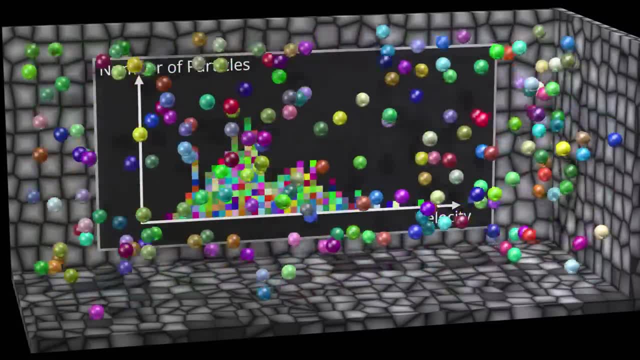 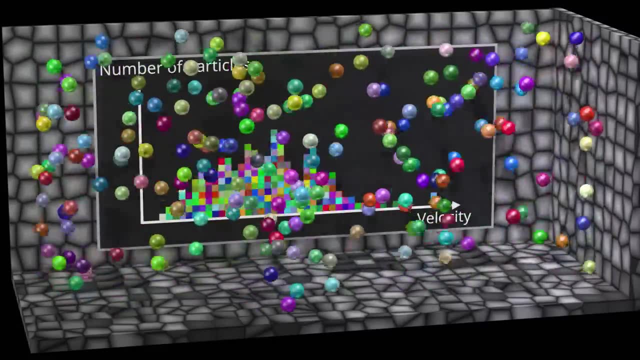 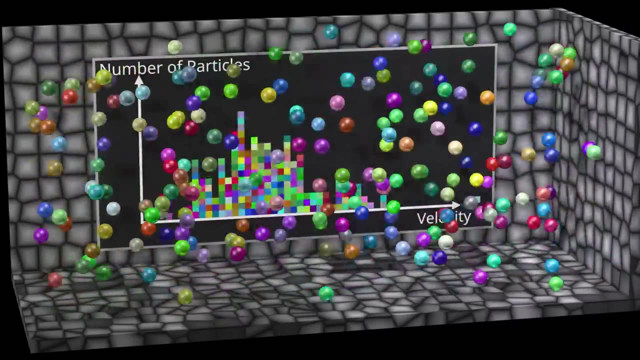 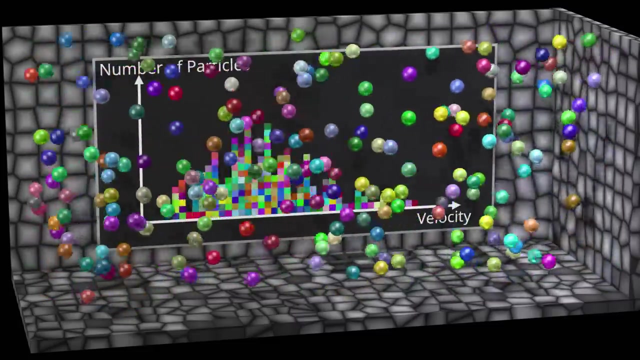 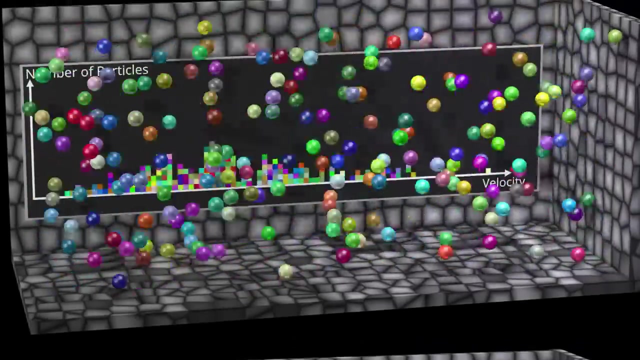 The total energy of the entire system is always constant. The average kinetic energy per sphere is what we call temperature. If we increase the temperature by adding energy to the system, the graph for the velocity distribution changes as shown. If we increase the temperature by adding energy to the system, the graph for the velocity distribution changes as shown. 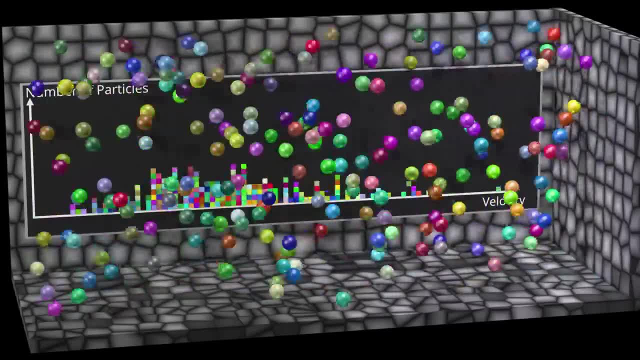 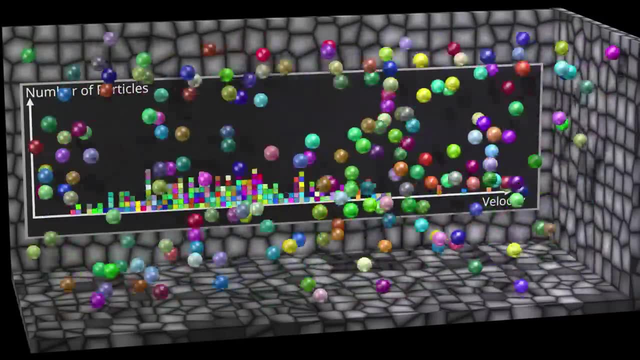 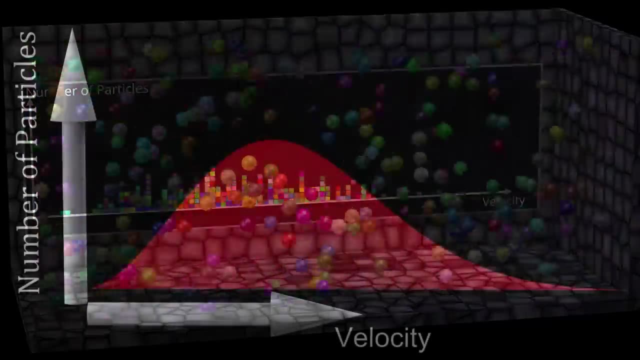 This system now has a higher entropy than before because with more energy, there are more different ways in which the energy can be distributed. If we increase the temperature by adding energy to the system, the graph for the velocity distribution changes as shown On average. the graph will look like this: 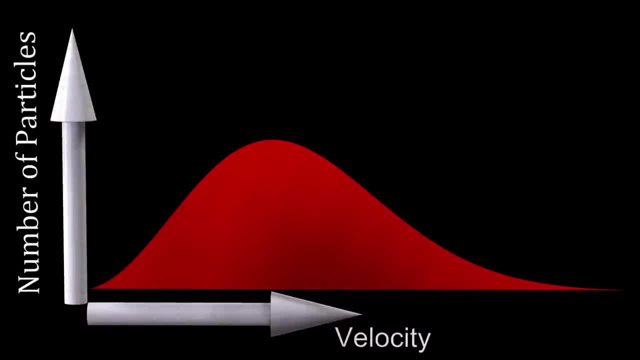 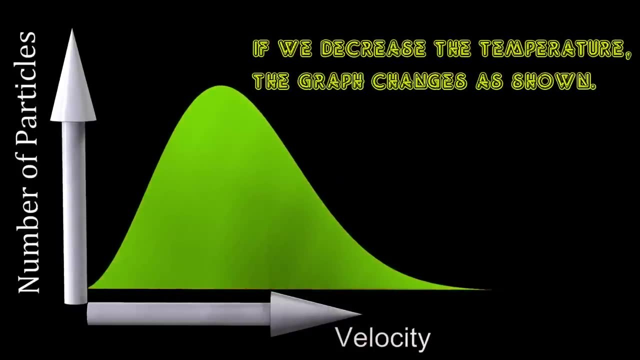 If we increase the temperature by adding energy to the system, the graph for the velocity distribution changes as shown. If we decrease the temperature, the graph changes as shown. If we increase the temperature by adding energy to the system, the graph for the velocity distribution changes as shown. 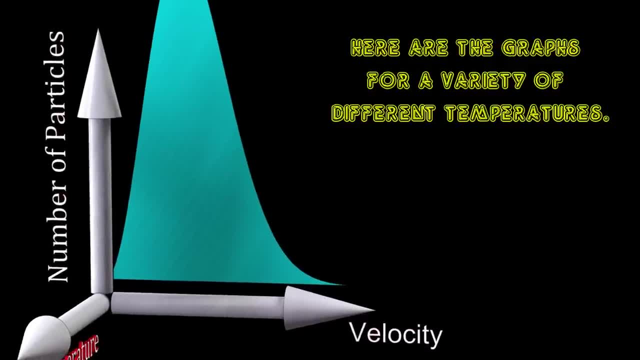 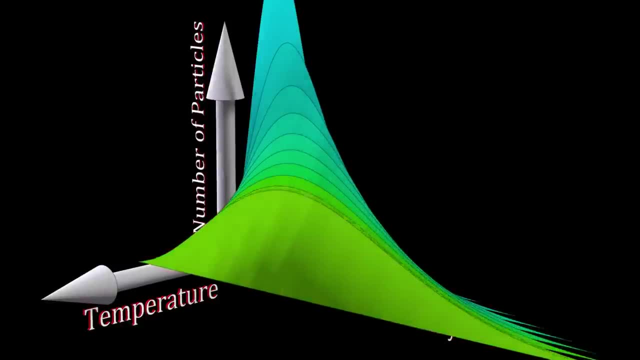 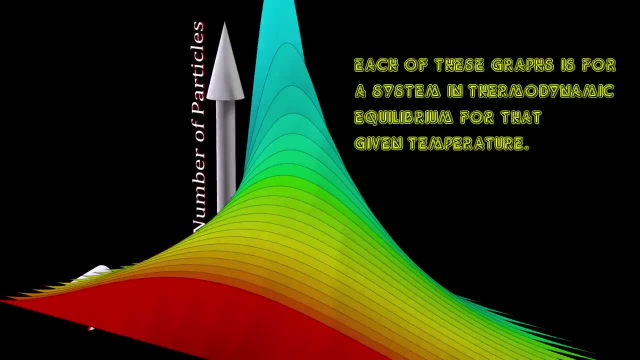 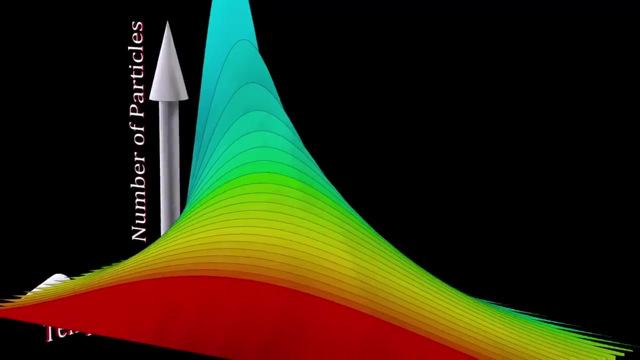 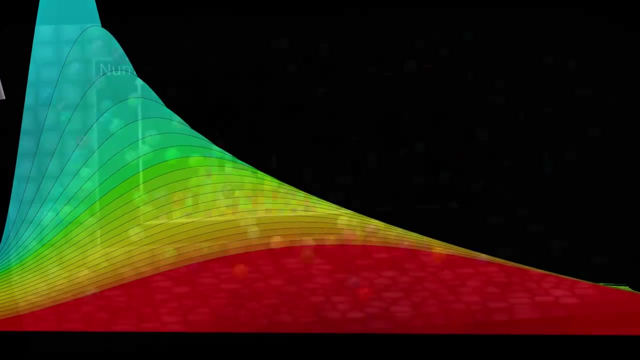 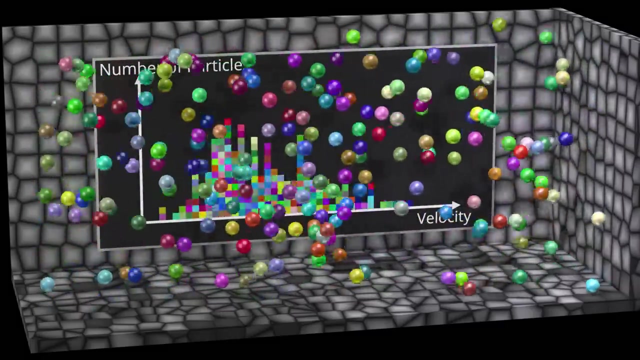 Here are the graphs for a variety of different temperatures. Each of these graphs is for a system in thermodynamic equilibrium for that given temperature. A system is in thermodynamic equilibrium when the entropy of the system has reached its maximum possible value. given the constraints of the system, 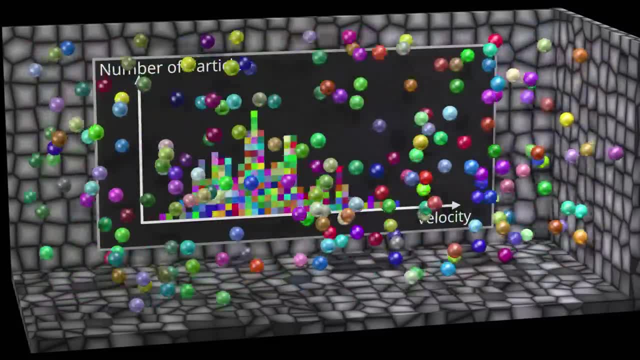 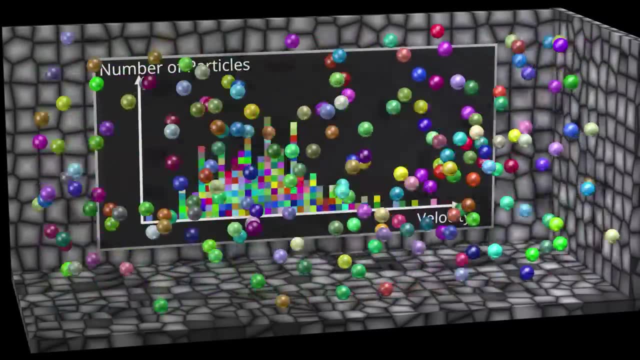 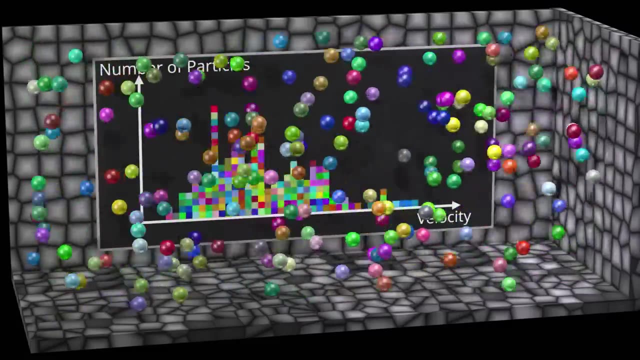 Entropy is a measure of how many different ways something can occur. Each of the different ways something can occur is what we call a microstate. Here, a microstate would consist of all the positions and velocities of all the particles at a given moment in time. 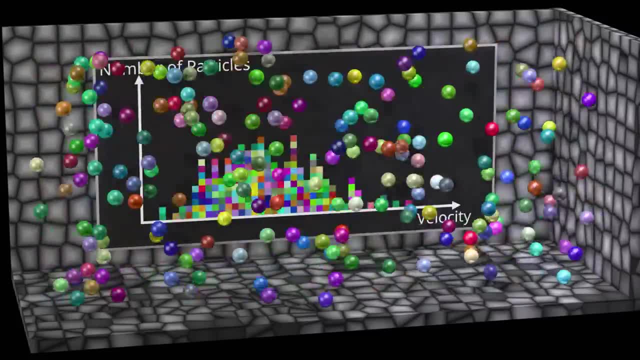 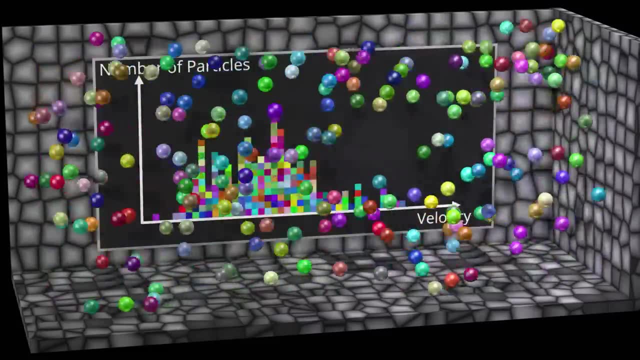 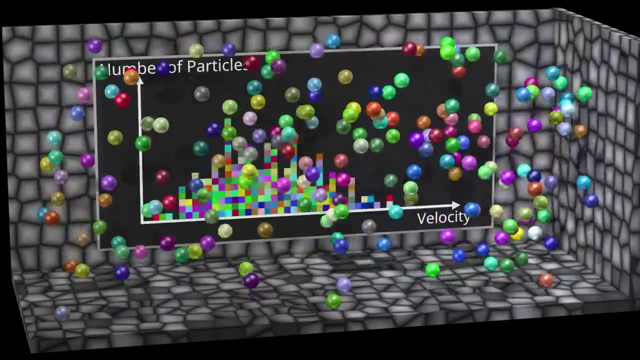 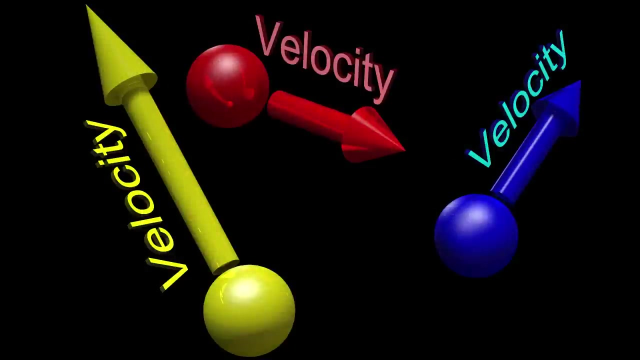 In quantum physics the way we count microstates is different than in classical physics. For example, consider the positions and velocities of several identical particles at a given moment in time. Now consider a situation where we have the exact same set of positions and velocities, but we swap the colors of the particles. 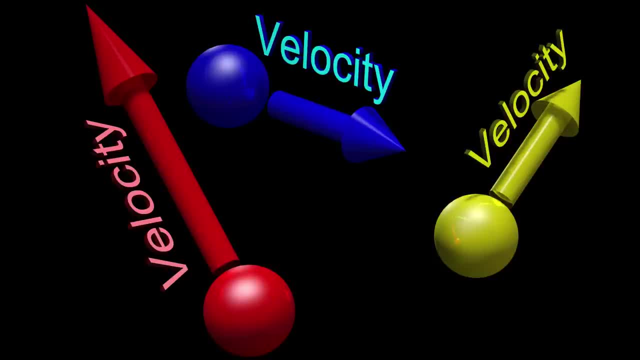 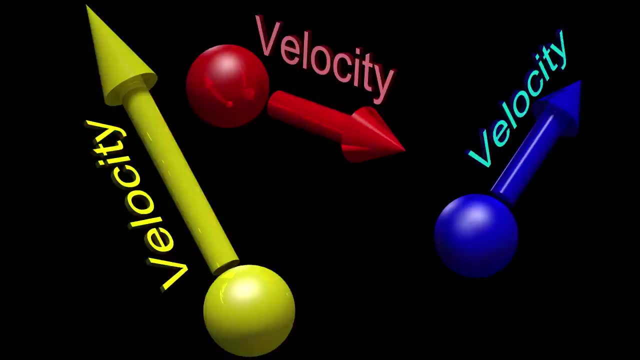 In a classical system we can do this because the particles are distinguishable and each of these cases is counted as a separate possible microstate. However, in a quantum system, identical particles are indistinguishable and therefore all these cases are counted as only a single possible microstate. 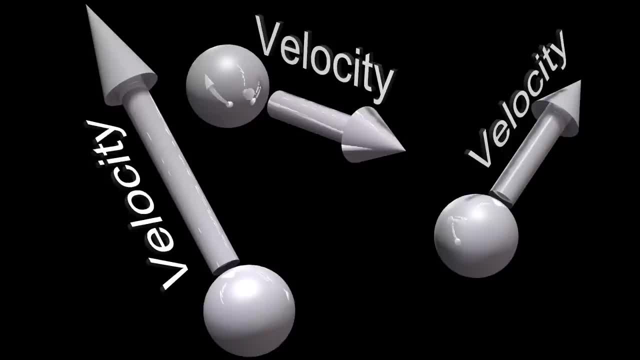 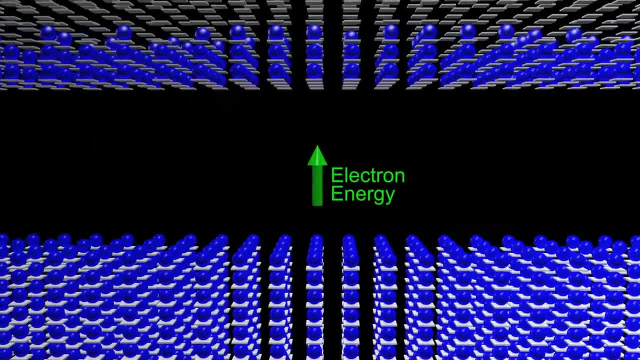 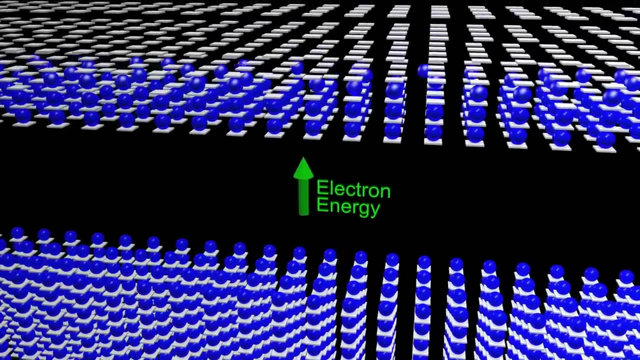 Hence the thermodynamic equilibrium is different for a quantum system than for a classical system. Also, in a quantum system, the thermodynamic equilibrium is different depending on if we are dealing with particles such as electrons, which obey the Pauli Exclusion Principle.